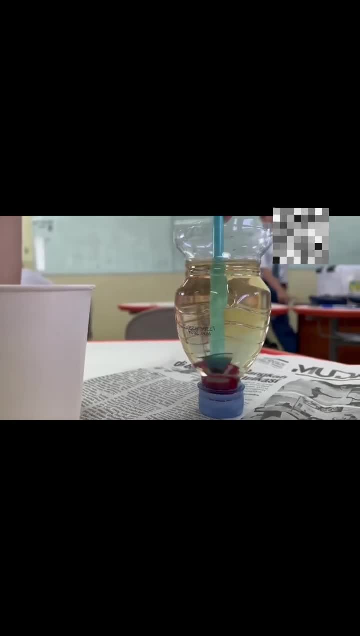 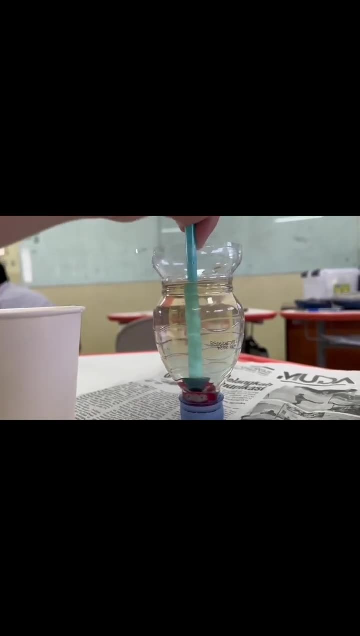 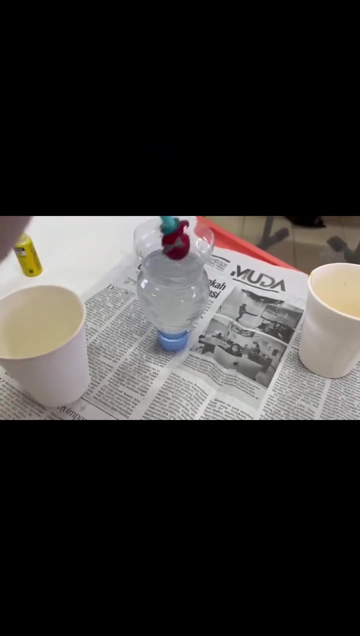 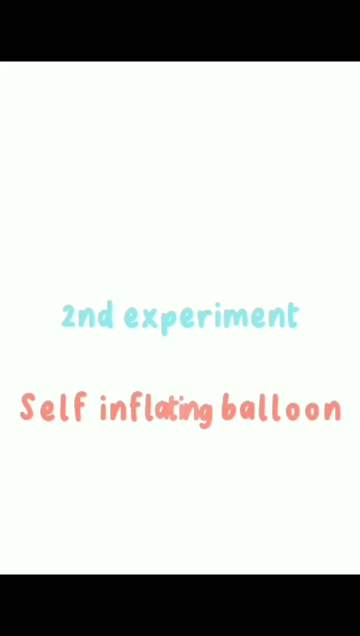 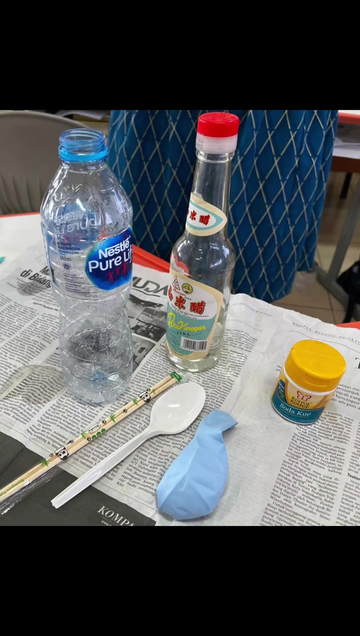 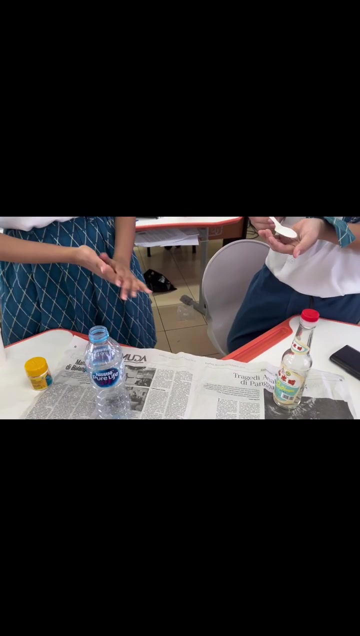 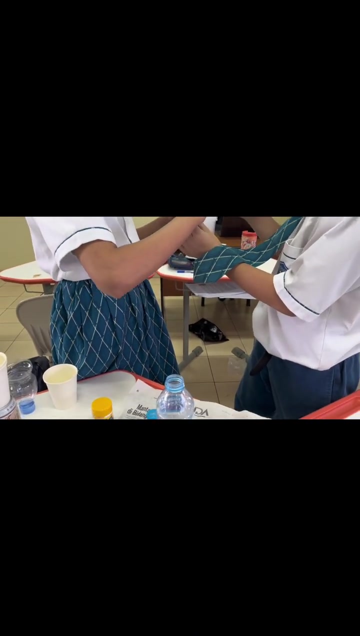 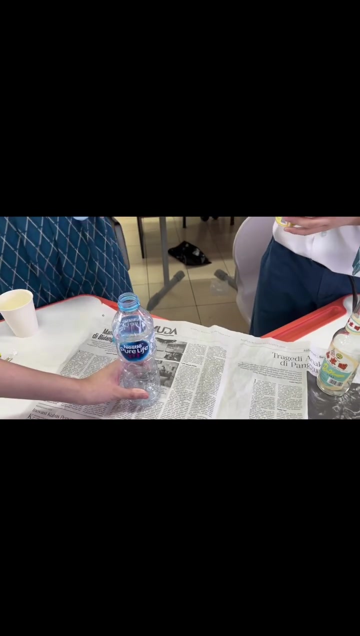 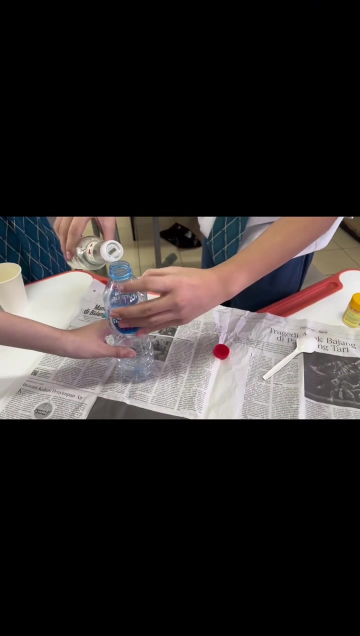 Hey, it's transparent, Self-inflating balloon. Prepare your ingredients: Vinegar, baking soda balloon, a spoon and an empty water bottle. First, we put the baking soda in the balloon with a spoon, Then pour your vinegar into the empty water bottle. 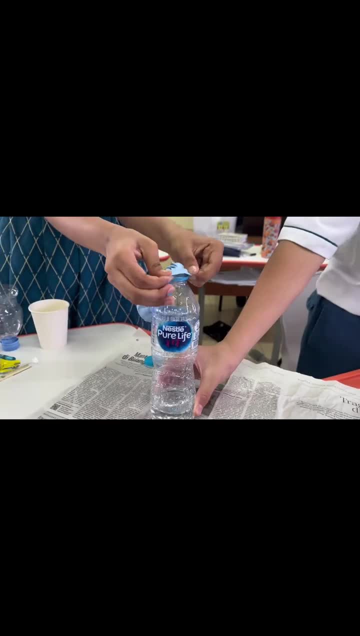 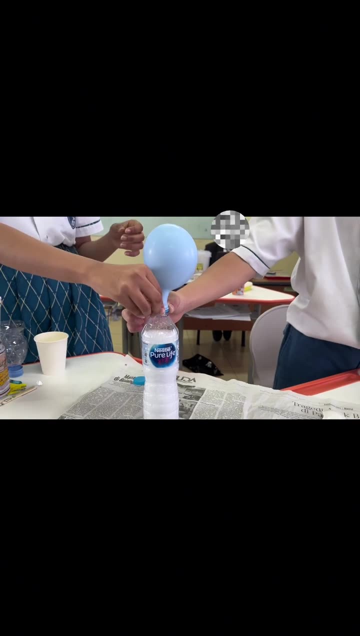 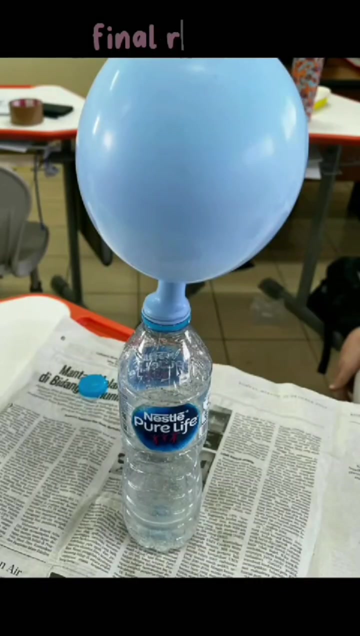 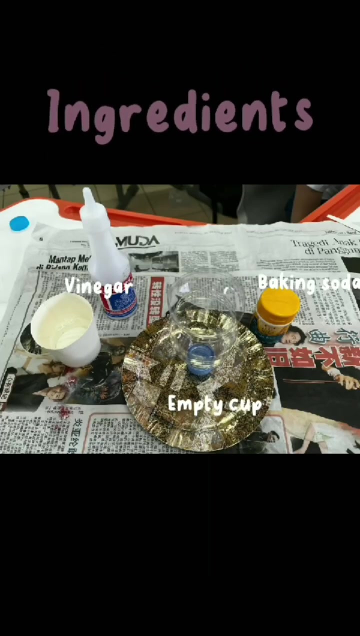 And finally attach your balloon onto the tip of the bottle. 3,, 2,, 1.. Tada, Final result. Final experiment: Baking soda and vinegar, Vinegar, empty cup baking soda and a paper plate. 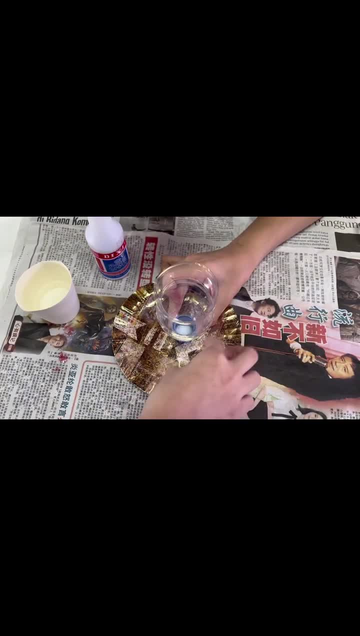 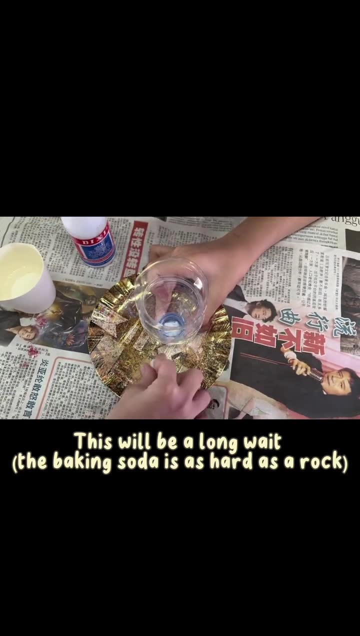 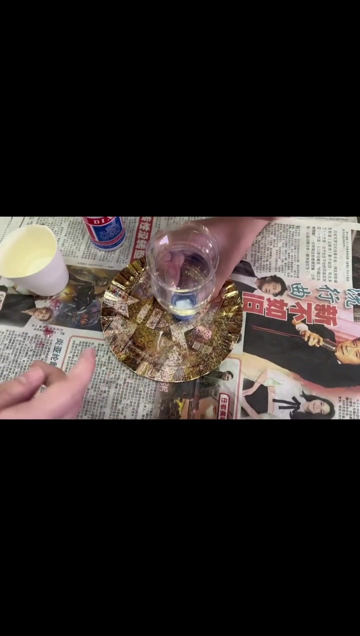 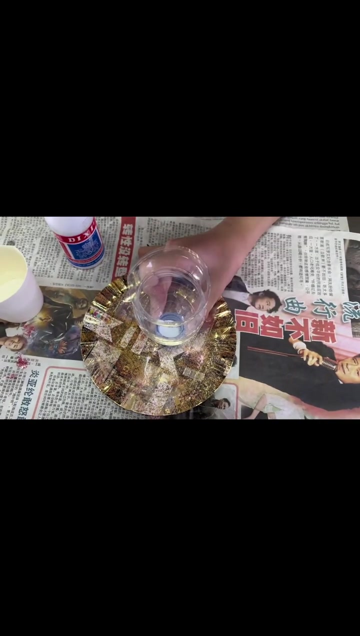 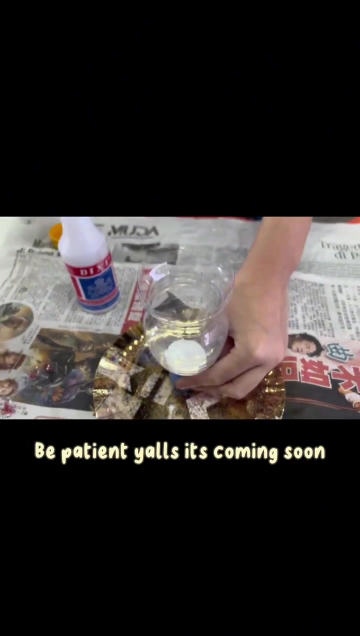 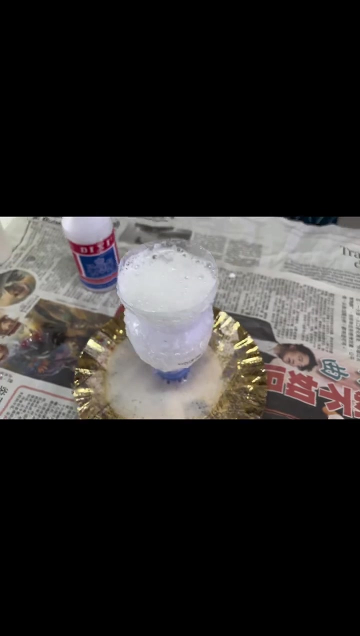 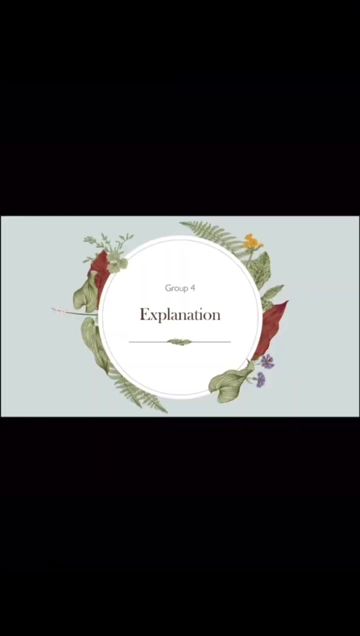 First, add your baking soda onto the empty cup. I'm sorry, but we're using your baking soda, Not your mom, Not your mom, Not your mom. It's broken. then pour your vinegar 3,2,1, And this is the explanation for our experiment. 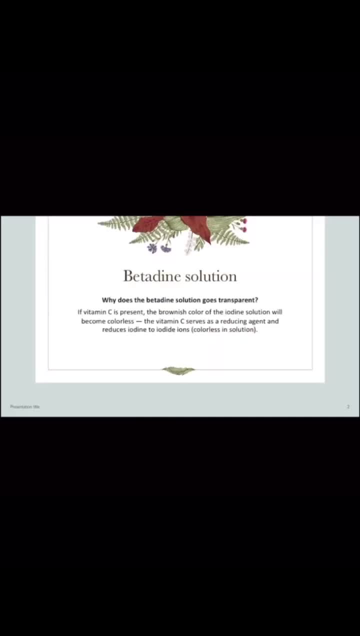 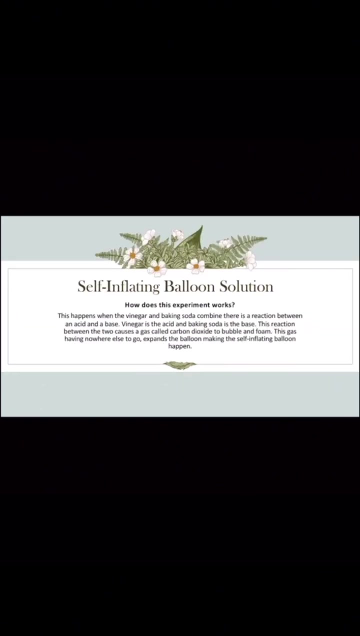 Let's start with the first explanation. Get that in solution. Vitamin C is present in the brownish color of iodine, Solution will become colors. The vitamin C serves as a reducing agent. Reduce iodine into iodide ions. Colors in the solution: Self-inflating balloon solution.